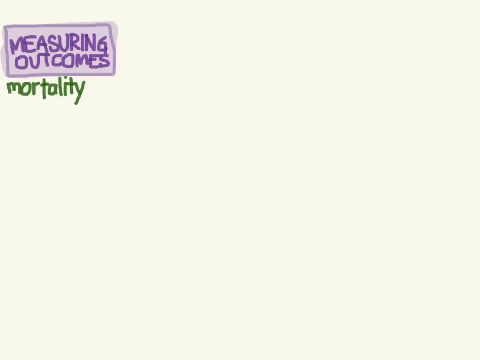 Let's continue with our conversation about mortality, and in the previous video we were looking at crude mortality rates, but in this one we're going to go to more specific ones. So instead of looking at the mortality rate for the entire population, as we did in crude mortality rates, maybe we want to break these guys up into certain groups, say like by age. 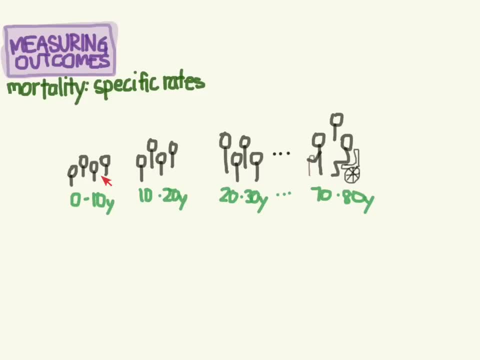 So we split up the population into various groups, like here: we've got 0 to 10-year-olds, 10 to 20s, 20 to 30s, etc. etc. and we've got our older population here, 70 to 80 years old, and then we can calculate mortality rates for each one of these groups. 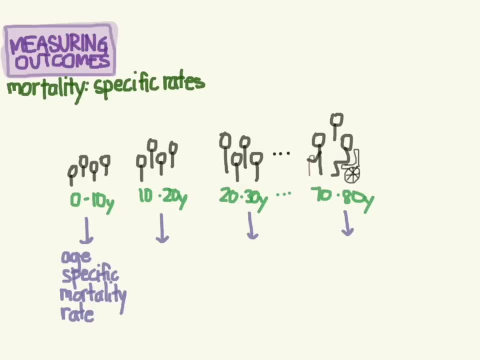 So for this first young group we calculate our age-specific mortality rate, the same for the next group and the next and the next, And so now we have We have various age-specific mortality rates, and the formula for this is very similar to the one that we had with the crude mortality rate. 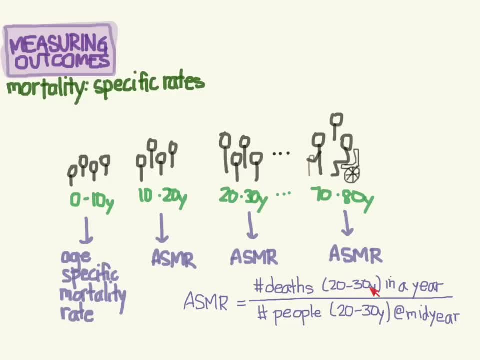 And so we have the number of deaths in the particular age group we're looking at in a year over the total number of people in that age group at mid-year. And so one thing that we really should stress here is that whatever criteria you're applying to the numerator, you better apply it to the denominator here as well, so it should apply to both. 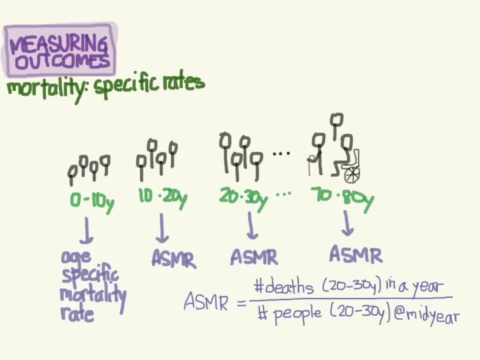 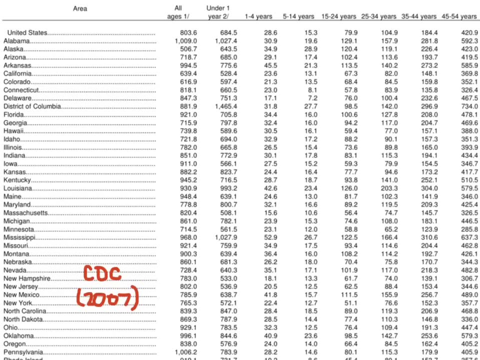 So let's take a look at an example, and this came off of the CDC website, and these are 2007 numbers, And so what we see here are the age-specific mortality rates, And so this first one, it's marked all ages, so this is the mortality rate for all the states per 100,000 people. 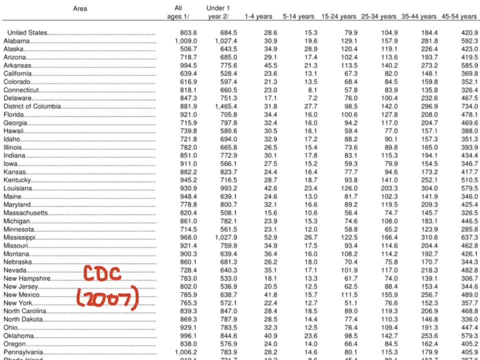 So it's not per 1,000.. Before it's per 100,000 people. So in 2007, in the United States, in total 803.6 people died per 100,000 people And if you look through at least what's listed here, the state that seems to be faring worst is Alabama. 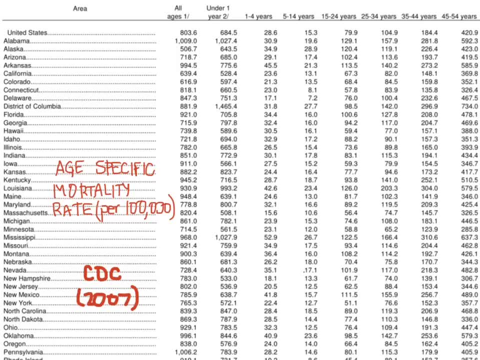 Now we break it down into various age-specific groups as well, So this one is the under 1 years old. These are the 1 to 4-year-olds, 5 to 14-year-olds, 15 to 24,, 25 to 34,, 45 to 54, and 55 to 64.. 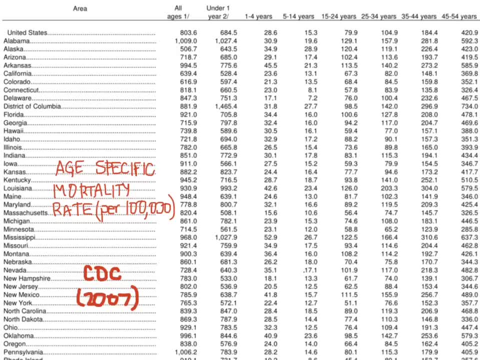 It continues onward, but I just couldn't fit it all on the screen And so now you can compare the various age-specific mortality rates in the various states. So we could look at. let's look at the infant mortality rate, which is the mortality rate in those less than a year of age. 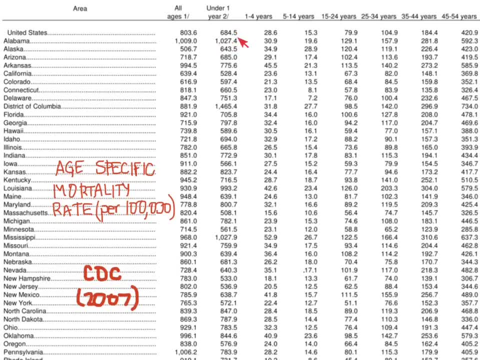 So look What states are not doing so good. Alabama's not doing so good. What is this one? This is DC. Wow, I wouldn't have guessed that DC would be so bad. And what's this one here? 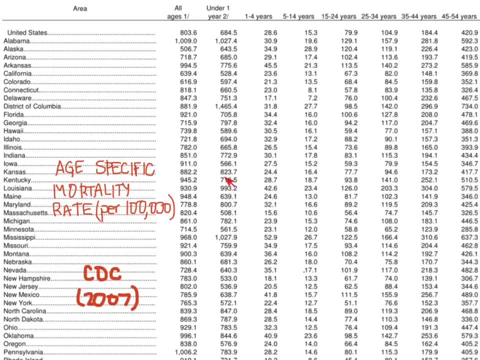 Mississippi. Yeah, that seems about right, And so you could see that the mortality rates for infants, the infant mortality rate here, and you can compare the various states. And then we've got the older kids here and we keep going in 10-year increments on up over here as well. 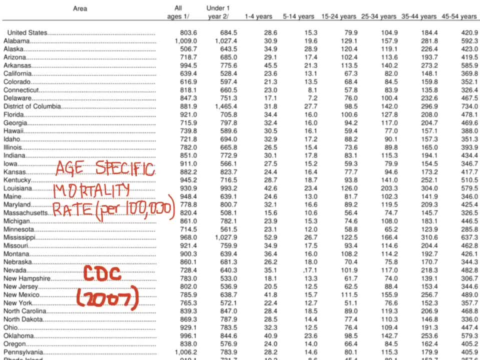 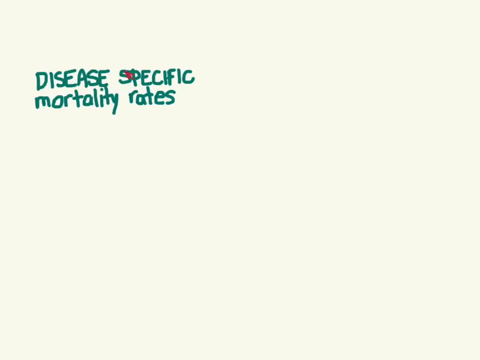 So these are age-specific. These are the age-specific mortality rates, and just as we separated the groups out by age, we can also separate it out by disease and have disease-specific mortality rates, which are also known as cause-specific mortality rates. So an example of this would be: let's take a look at lung cancer. 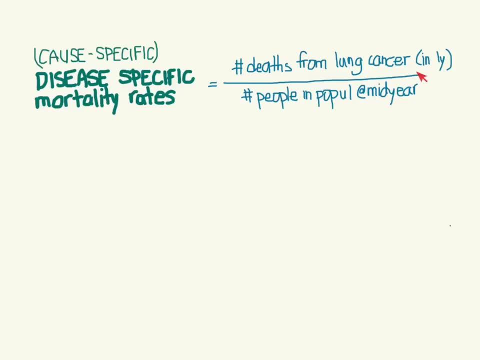 And so the formula would be the number of deaths from lung cancer in one year over the total number of people in the population At mid-year, and we'll probably multiply this by 1,000 as well, And this is a good way for comparing the mortality between two time periods. 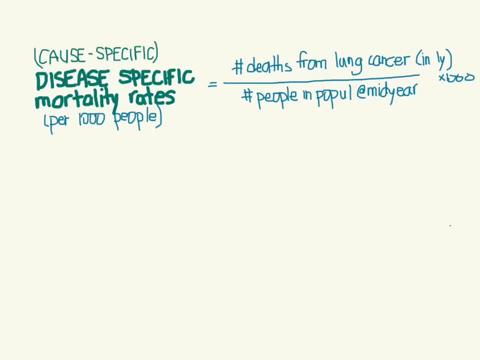 So you could say: what is the mortality for lung cancer in 1970, and let's compare it to 2010.. Now, one thing you should notice is the denominator here. Now, when we look at age-specific rates, we had the age up here and the age down here as well. 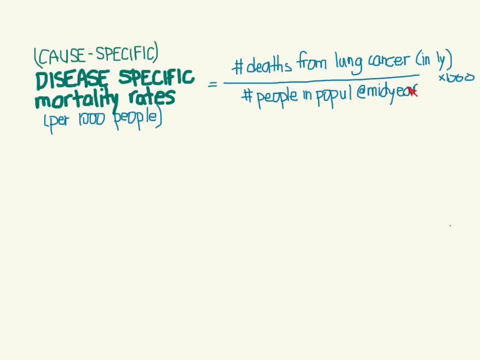 But we don't have that here. We have lung cancer, We have lung cancer here and the entire population here. So what if we made it different? What if we did this? And so instead we have the number of deaths from lung cancer in one year over the number of people with lung cancer at mid-year. 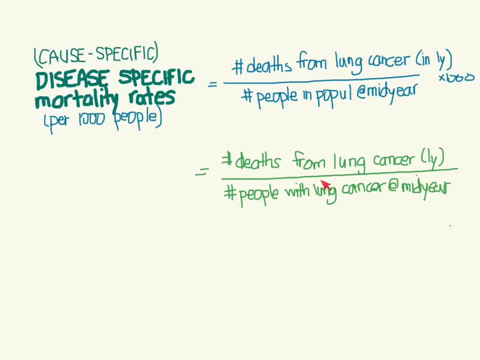 So you see the difference here. Here we have in the denominator people with lung cancer and here we have the number of people in the population, And so this is the difference here. the width lung cancer changes our denominator. Now, this is something we've actually looked at. 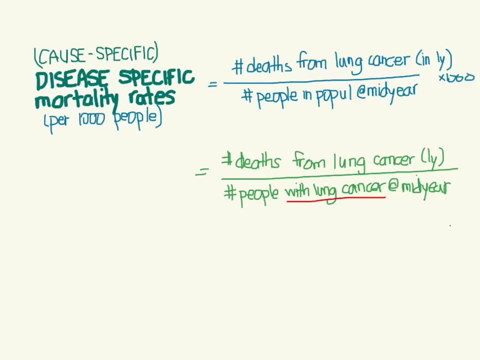 We looked at this in the incidence video and this is called the case fatality rate, with patients with lung cancer being the cases and death by lung cancer, of course, being the fatality. And so what this is? this is more of a measure of the severity of disease, and you can use it to compare other diseases. 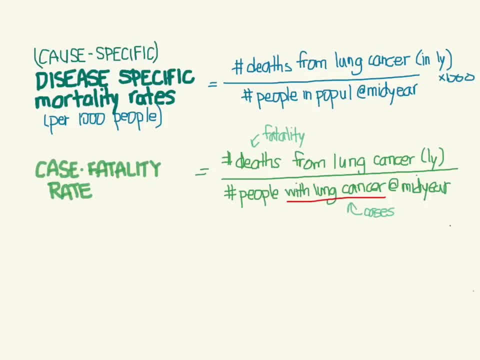 So you could compare the case fatality risk rate of lung cancer to say pneumonia and you might say, hey look, lung cancer. It has a much higher case fatality rate. It is much more deadly than pneumonia is. So disease-specific mortality rates we can use to compare how a disease is doing across time and case fatality rates we can use to compare the severity of a disease and we can use it to compare to other diseases. 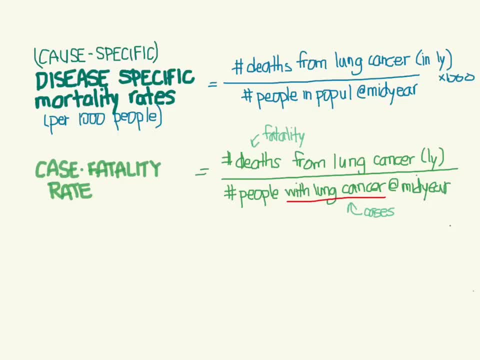 Now there's one more thing that we could put in the denominator. We'll have the numerator be the same thing: number of deaths from lung cancer in one year. But now in the denominator We'll put the number of total deaths, and what this is called is proportionate mortality. 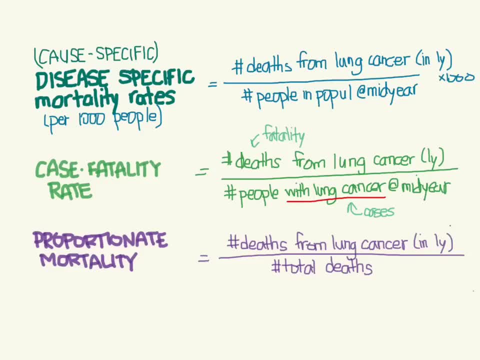 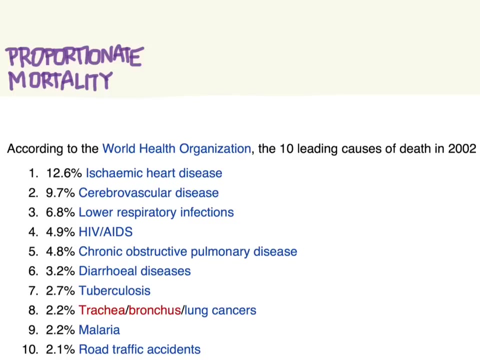 Basically what you're saying here is: of all the people who died in 2012,, how many of them died of lung cancer? What proportion of them died of lung cancer? So let's take a look at a quick example of this. So again from my favorite Wikipedia site on mortality: 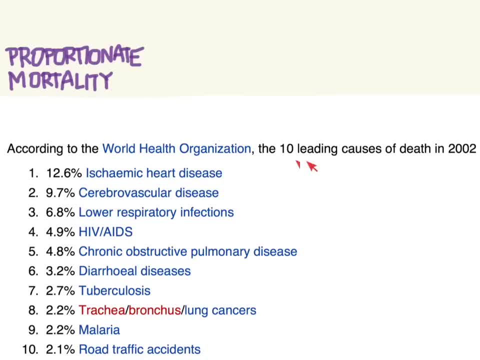 Mortality rates. I take another example, and here are the 10 leading causes of death in 2002.. And so, of all the people who died in 2002 in the world, according to the World Health Organization, 12.6% died of ischemic heart disease. 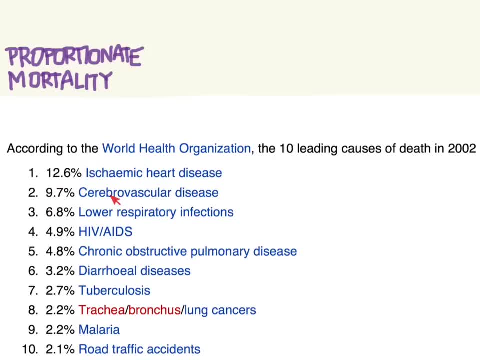 So they died of heart attacks, 9.7% died of strokes, 6.8% died of pneumonia, About 5% died of HIV Or AIDS, And so you can see this is the proportion of people that died of a certain thing.